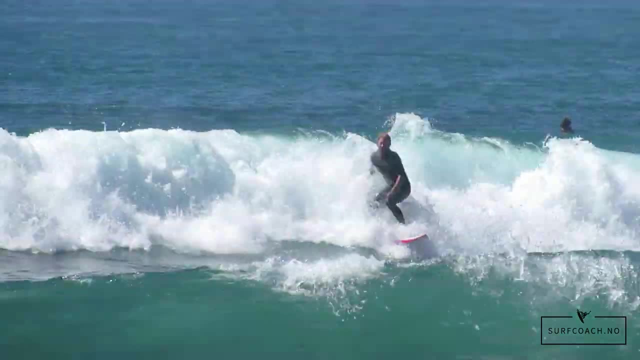 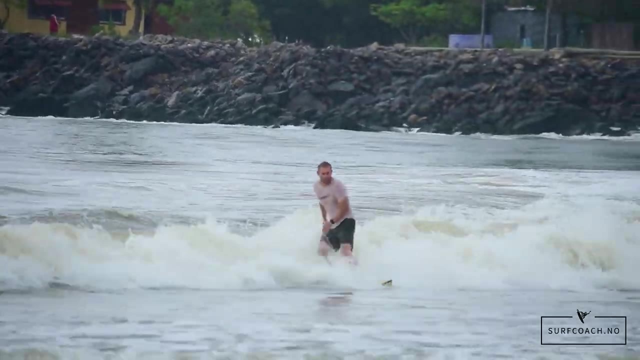 snaps. You can also do long lip-line floats or you can do some speed or projecting floats. You can also do some speed or projecting floats. You can also use the lip to do blow tails or airs or blow tail reverses. but it's not a good place for. 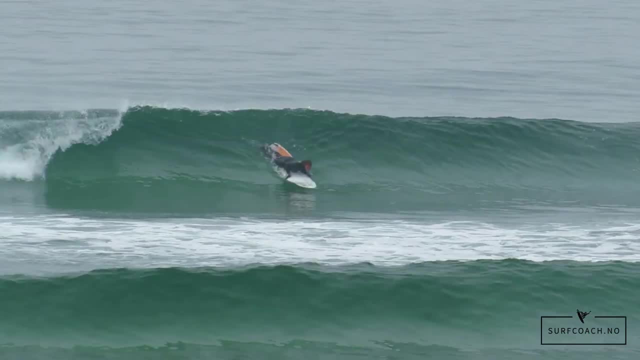 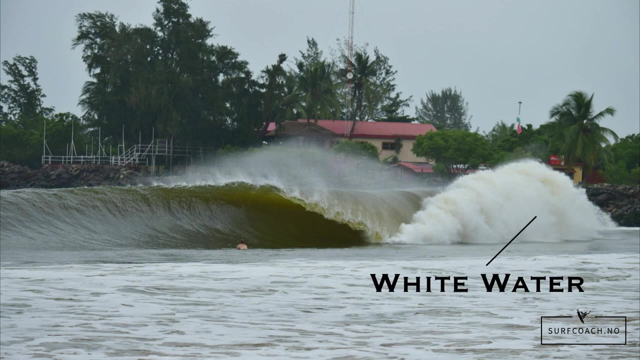 a beginner to try catch a wave at, because the lip is going to hit you pretty hard and you get slammed easily. That brings me to the next part of the wave, which we call the white water. The white water is the broken part of the wave, so once the lip has broken, it'll turn into a white water wave and that's. 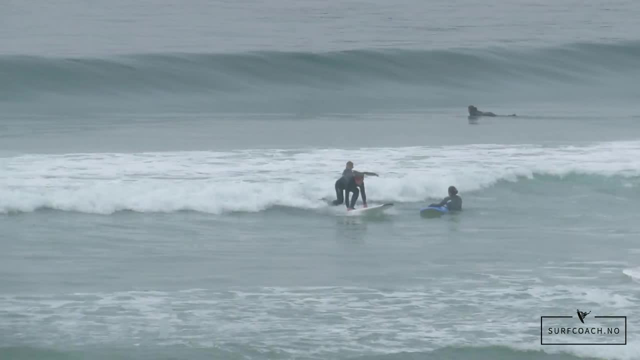 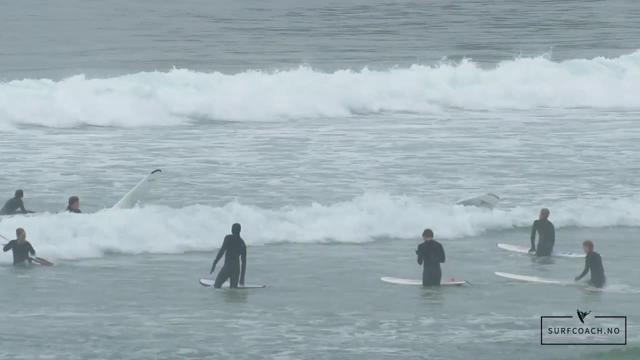 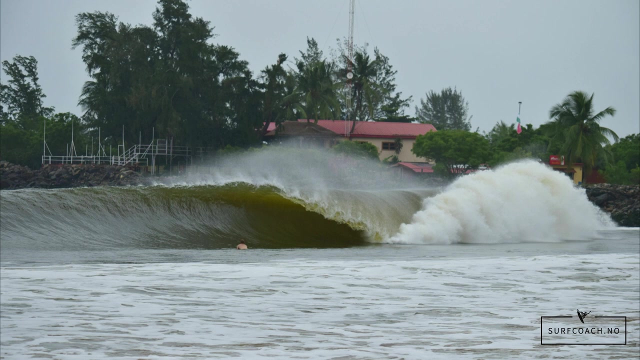 a really good part of the wave for first-time surfers or beginners to learn to catch the wave, stand up and surf without getting hurt and without too much struggle. When a wave hits a shallow sandbank or a reef, the lip is going to throw far away from itself. 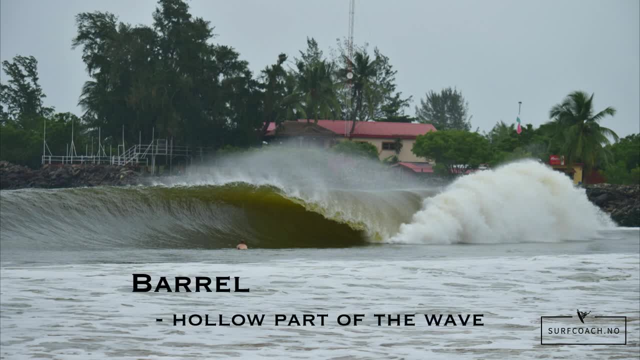 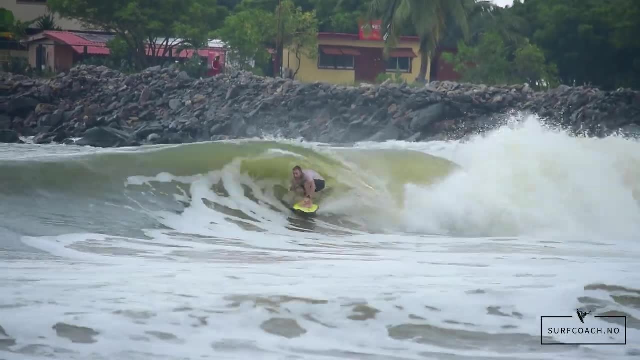 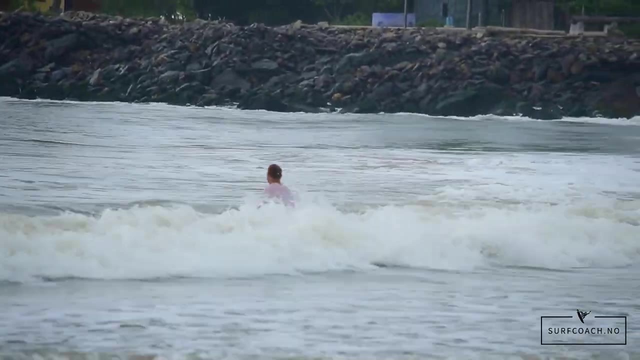 creating a hollow part on the wave, which we call a barrel. A barrel is one of the ultimate surf goals. That's a very cool, sensational feeling to be inside that hollow part and let the wave barrel and break over you. Sometimes you get a big barrel, sometimes small barrels, but a barrel is a barrel. 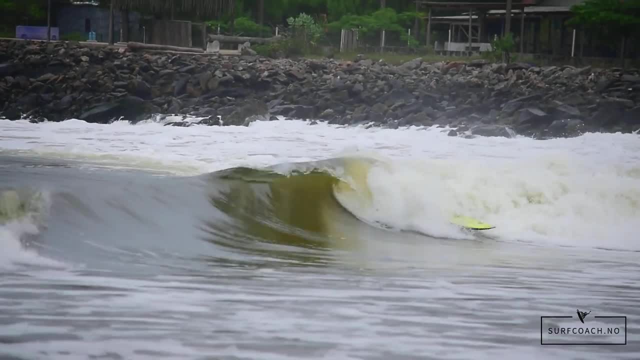 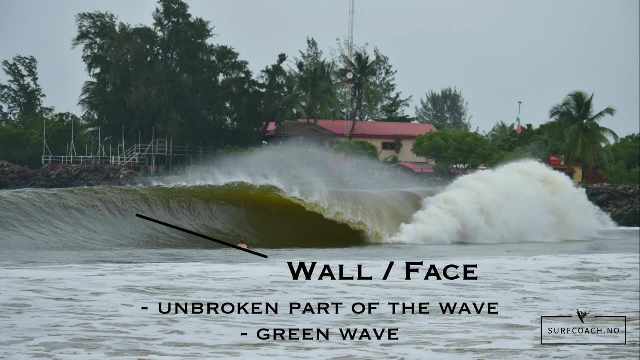 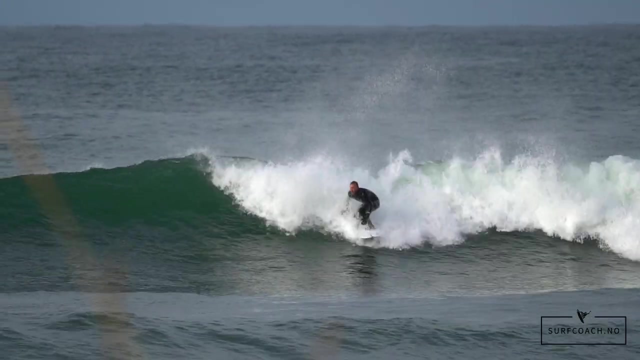 and it's always fun. Now, next to the lip of the wave, you have the unbroken part of the wave, which is also called the green wave, which we call in surfing, the wall, or the face, and this is the part of surfing you use to do turns. The wall and the face of the wave is going to have different parts. 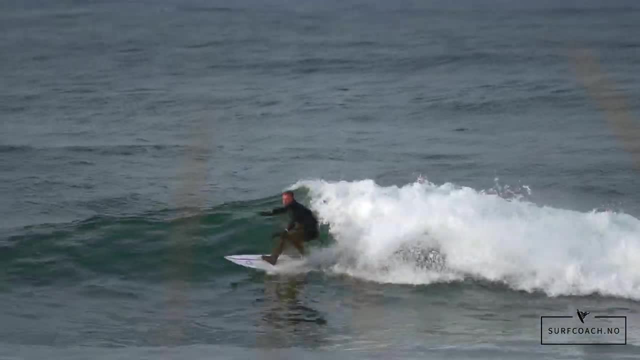 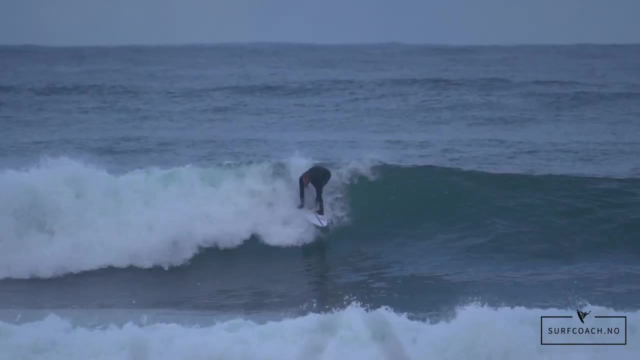 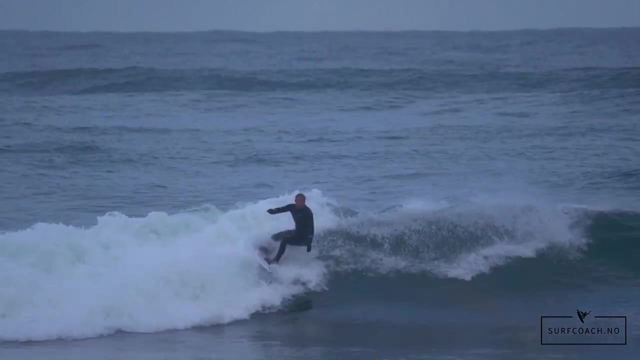 and each part is going to allow you to do different kinds of maneuvers. Some parts of the wall or the face of the wave will be steeper and more critical, and then other parts will be more gentle, a bit softer and slower. The wall or the face of the wave 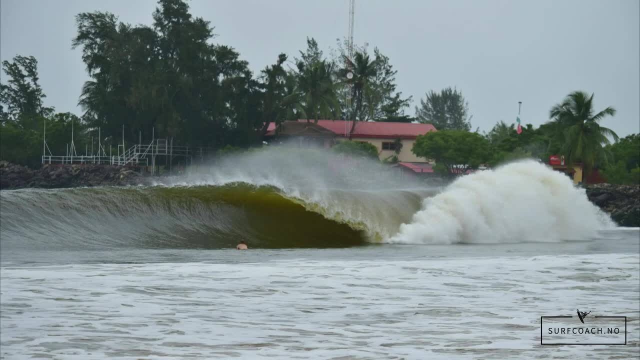 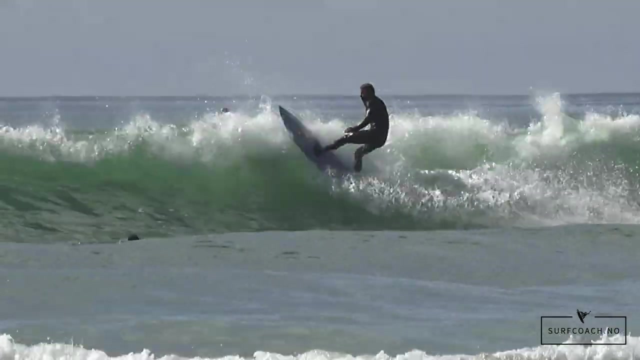 will have two different parts. The one part is the pocket and the other is the shoulder. The pocket is the power source of the wave and is a good place to keep and to find your speed and flow and a great place to do more radical and more critical maneuvers.